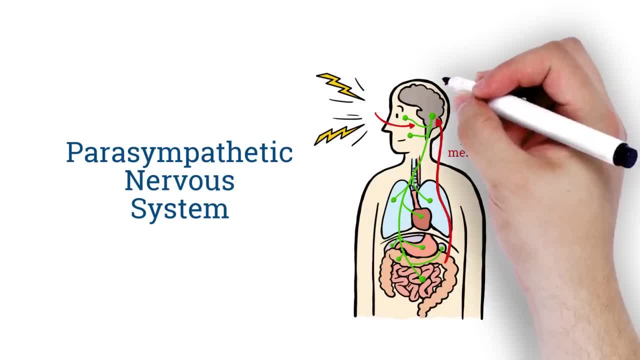 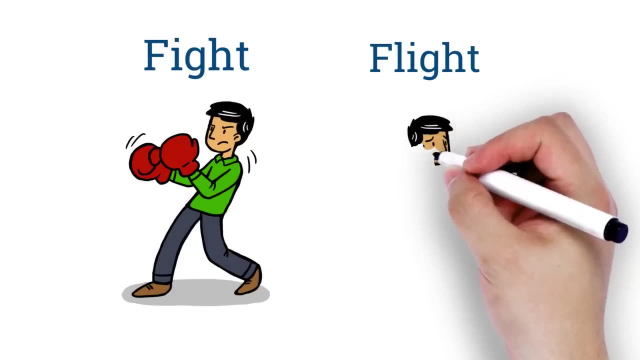 relaying messages from the internal and external sense organs to the brain, where subconscious decisions are made, whether to suppress or activate the sympathetic response. The sympathetic fight or flight reflex is constantly primed to rapidly respond to danger signals. This state is suppressed by the parasympathetic system. 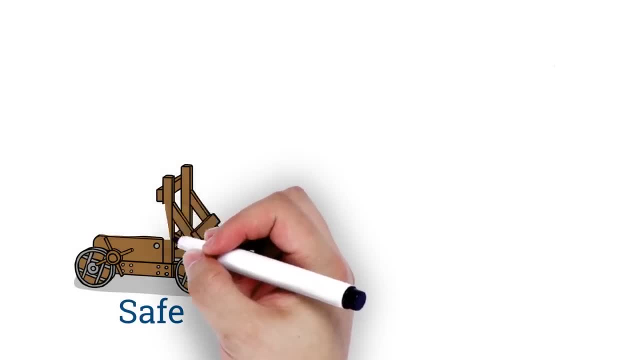 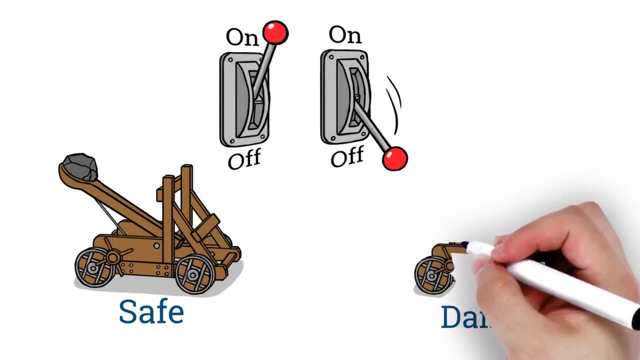 When conditions are interpreted as safe, the vagus brake is engaged to restrain the ever-repeating nervous system. The parasympathetic system is then re-engaged by the parasympathetic reflex. Any signal perceived as danger releases the vagus brake. 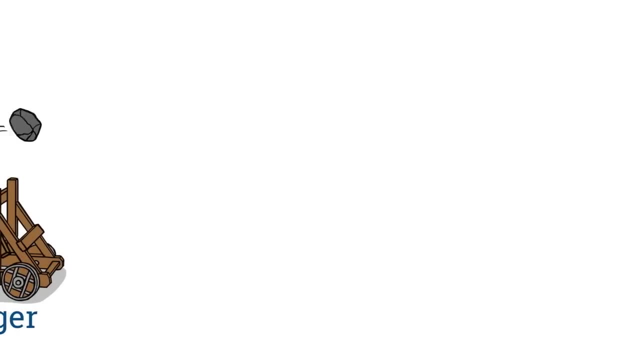 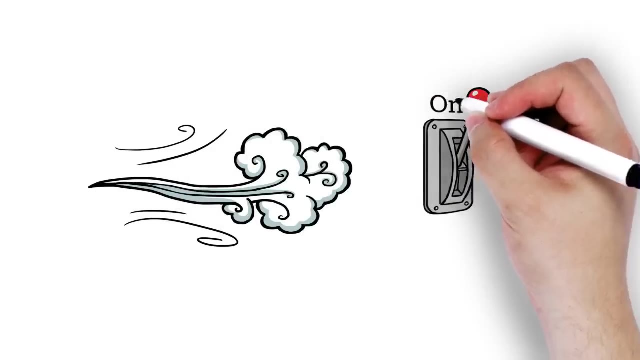 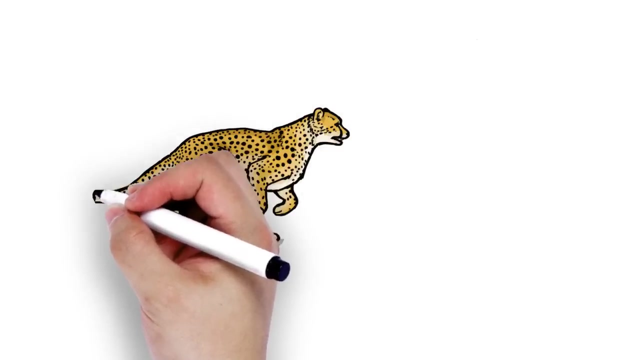 freeing the sympathetic response to activate. If the signal is recognized as just a rustle in the breeze, the vagus brake rapidly re-engages, allowing a period of calm to continue. If perceived as life-threatening, the vagus brake will fully disengage. 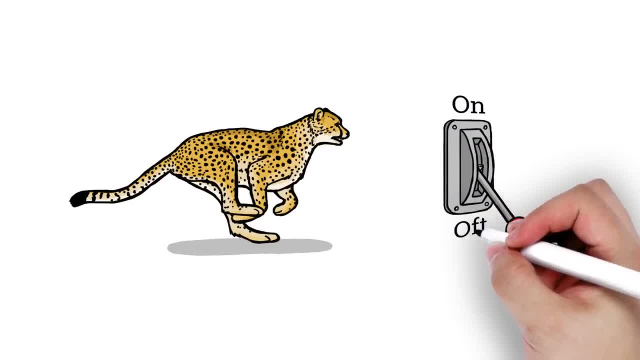 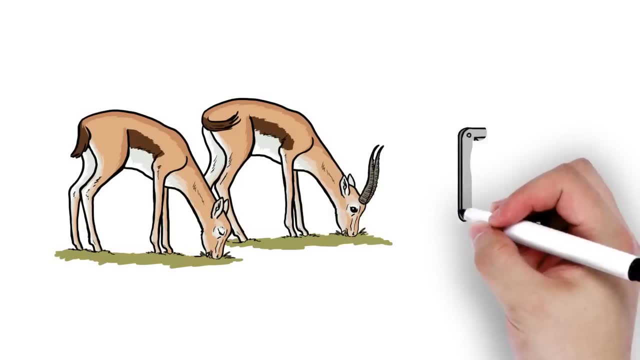 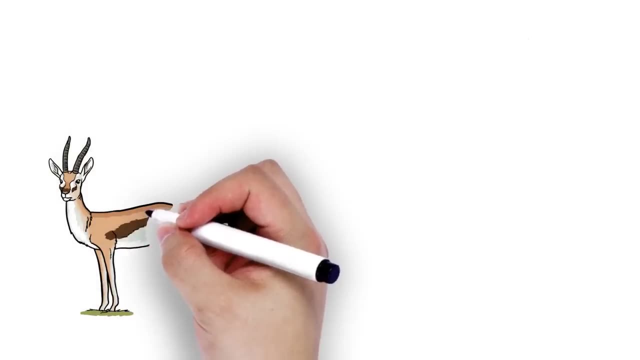 allowing sympathetic dominance to engage with the energy-consuming fight or flight response. If the danger passes, the vagus brake will re-engage, restoring a state of restfulness, energy replenishment and recovery In humans. the gazelle's anxiety about predators has been replaced by the stress of modern life. This sets the scene for abnormally prolonged and energy-sapping sympathetic activation, with diminished time for the parasympathetic dominance required for recovery. Parasympathetic and sympathetic imbalance is recognized as a significant factor contributing to both psychological and physical illness. 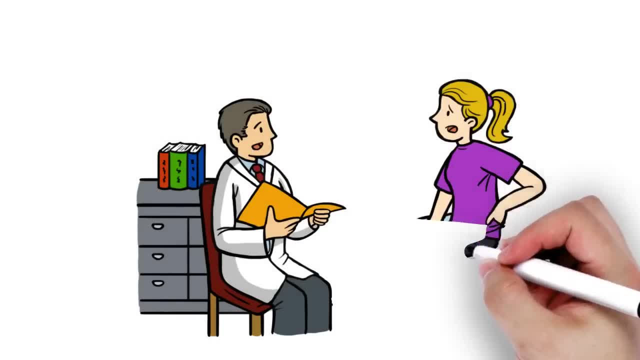 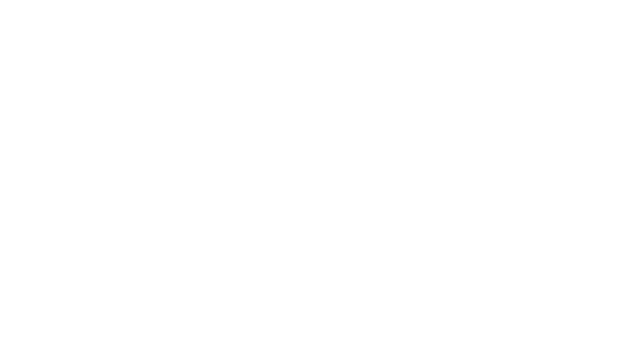 In the clinical setting. assessment of autonomic balance has been difficult to measure. What if there was an objective measure of sympathetic and parasympathetic balance? The phenomenon known as heart rate variability. HRV provides a window to these opposing systems. 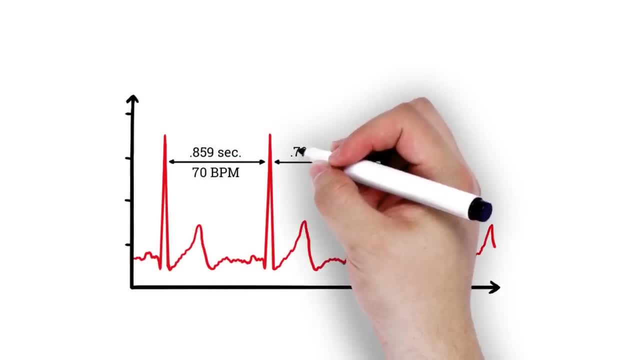 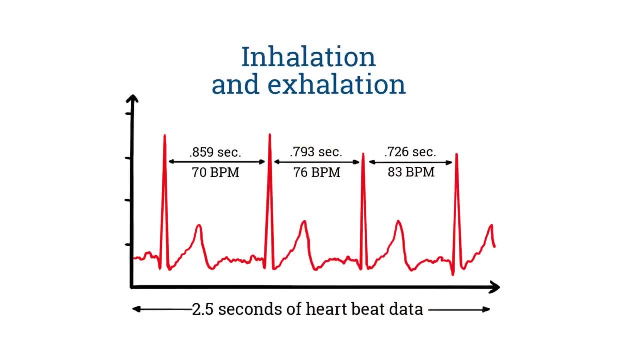 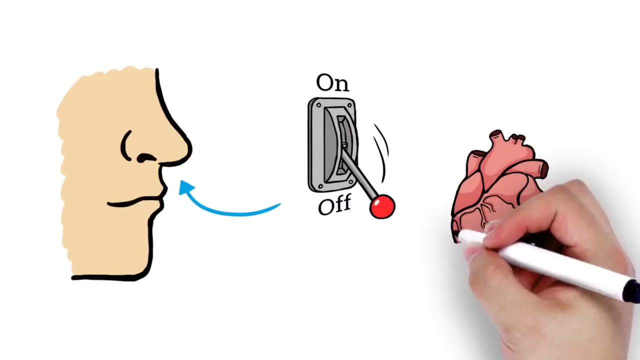 HRV reflects subtle changes in the duration of single heartbeats during inhalation and exhalation. This is regulated by vagus nerve connections to the heart. During inhalation, the vagus brake is briefly released, allowing a sympathetic increase in heart rate. 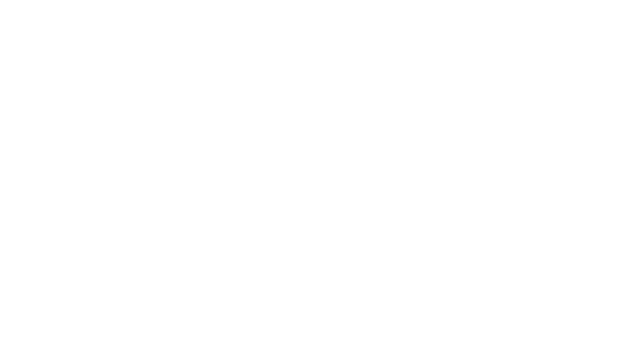 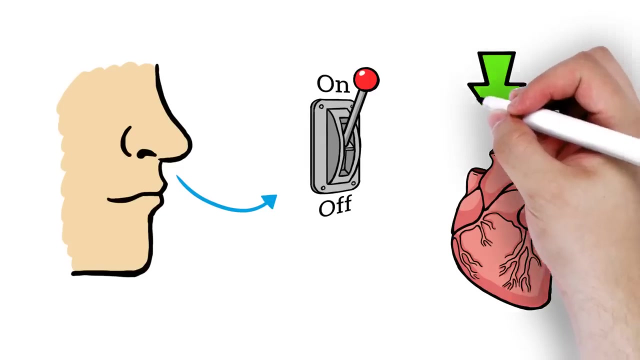 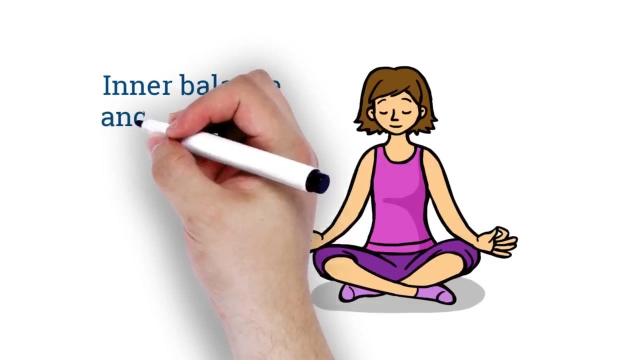 and decreasing the duration between each heartbeat During exhalation the vagus re-engages, slowing the heart rate and increasing the duration between each beat of the heart. Heart rate variability is normal and indicates autonomic balance and a state of inner balance and well-being.